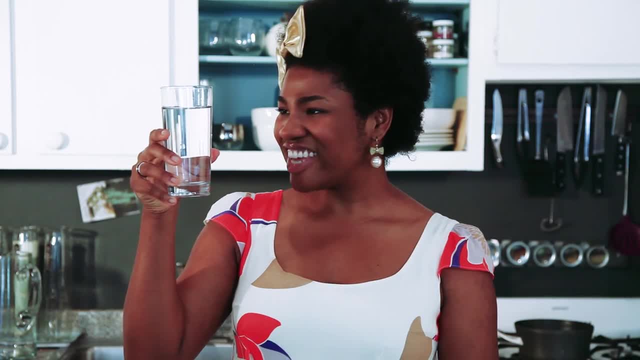 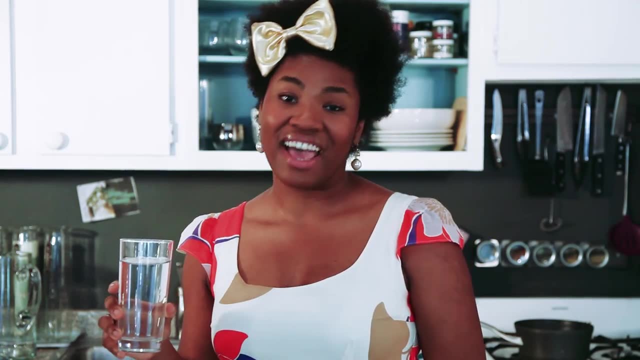 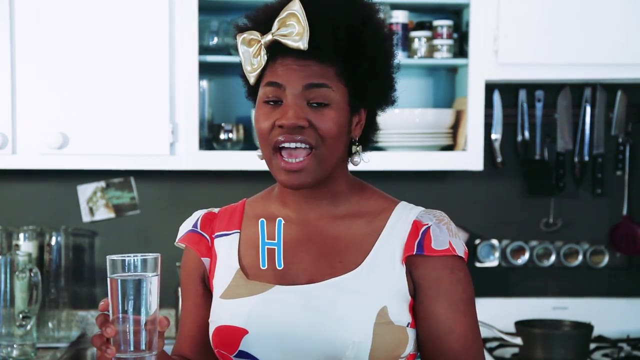 Take a look at it: Clear, beautiful, refreshing the sustenance of life. Now is the perfect time for me to tell you that water is actually made up of three atoms: A hydrogen atom, a hydrogen atom and an oxygen atom That makes up H2O, the molecular structure of water. 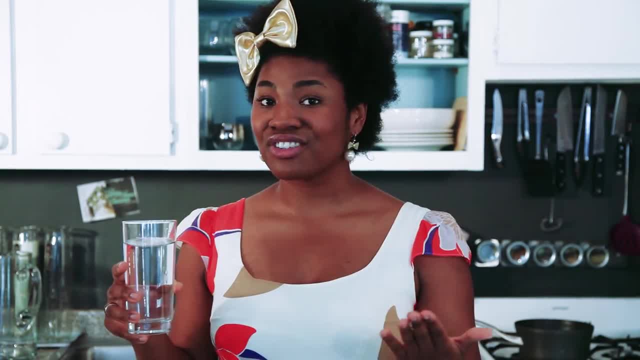 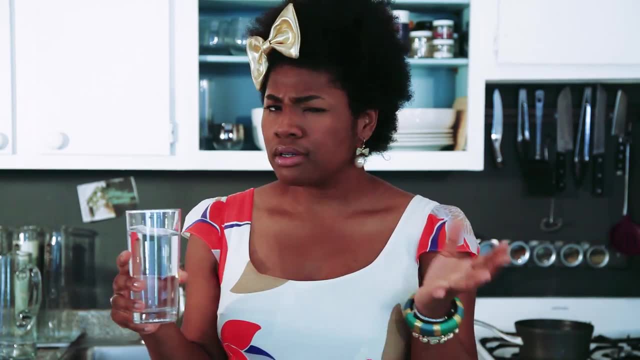 Now, this glass of water is room temperature, so the water is in its liquid form. So what we're going to do is pour ourselves a glass of water. The molecules in this glass of water are close together, but not packed super tight. They're moving all around each other, just kind of hanging out and thumping around. 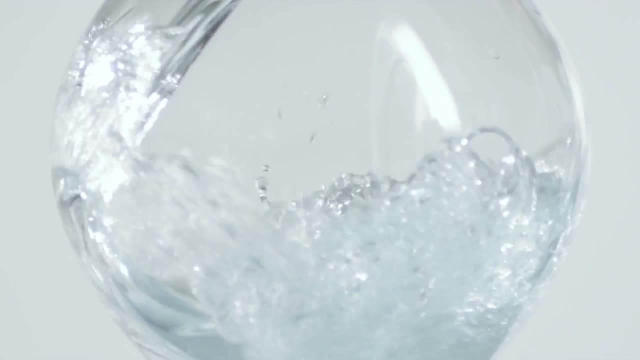 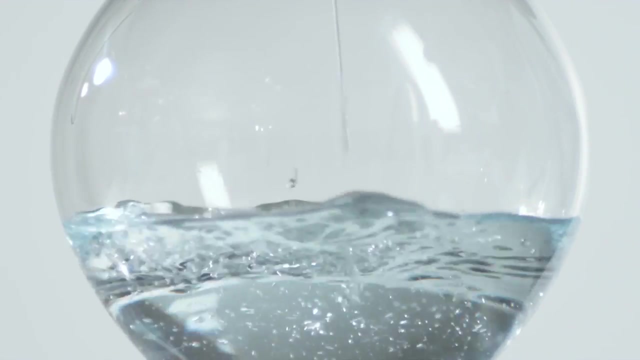 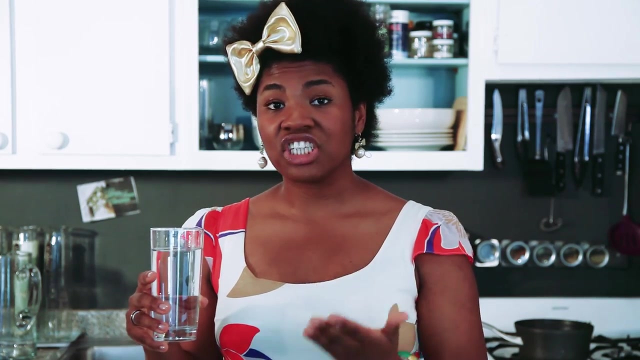 Now, liquids have no definite shape and they take on the shape of whatever they happen to be in. Some are sticky, some are gooey and some are just wet and run all over the place. Extreme temperatures like heat and cold is enough energy to change the states of matter. 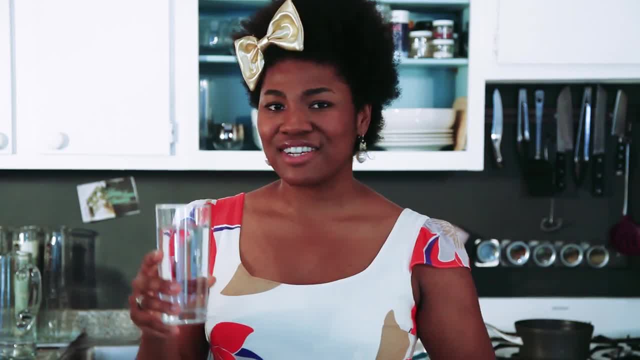 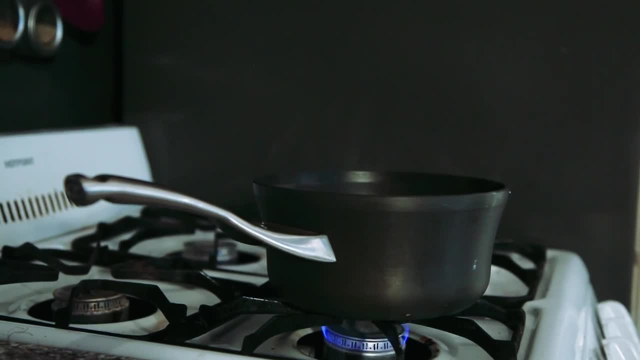 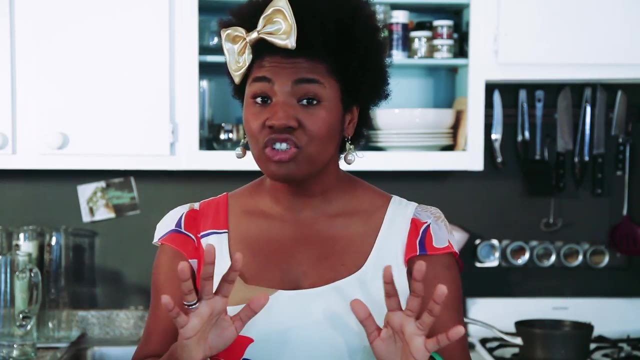 Take this glass of water and pour it into a pot, Turn the heat up and let's observe what happens. STEAM Gas Gas molecules want nothing to do with each other. They're flying all about at super fast rates. they take up no shape at all and no volume. 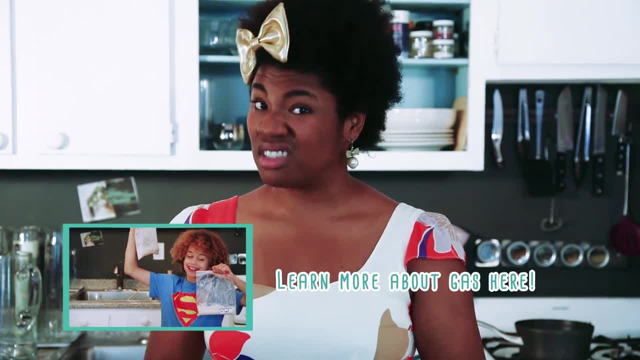 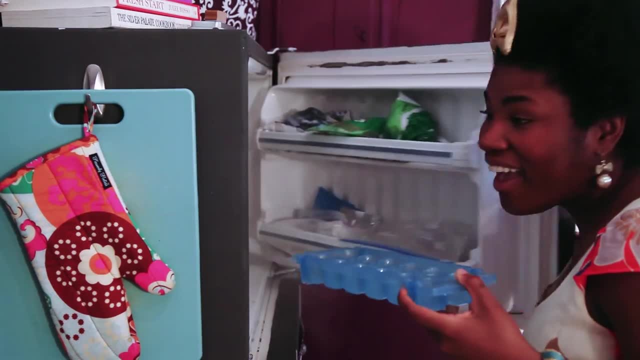 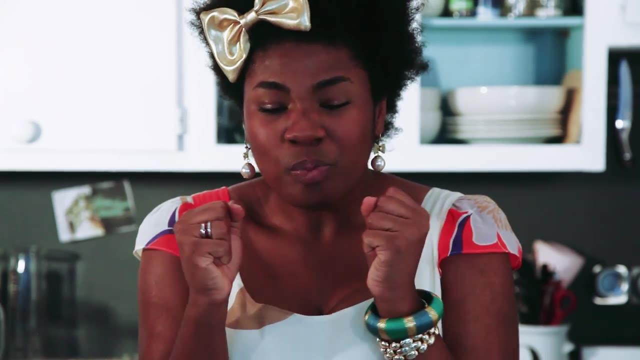 Now. you can't see gas usually, but sometimes you can smell it. Pour the remaining water into an ice tray, Pop it in the freezer and what do you have a few hours later? ICE. This is your solid Molecules, and solid are packed super tight and vibrate in a fixed position. 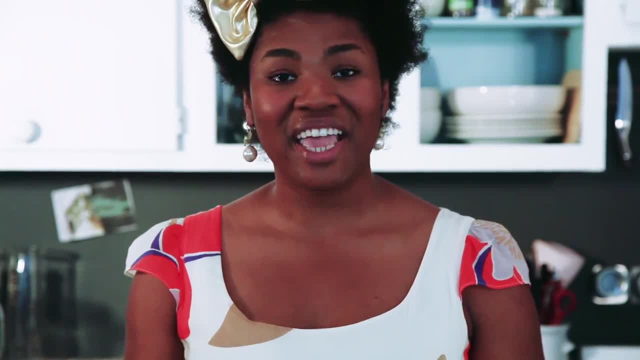 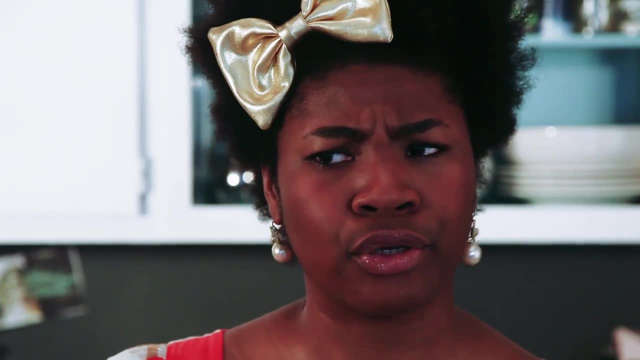 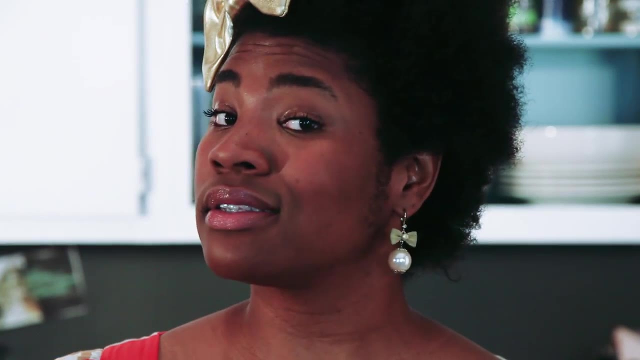 They have a definite shape and volume. measurable space an object or substance takes up, Not that volume. So there you have it, everyone the three states of water, But no matter what, it is all still just H2O. So the next time someone asks you, 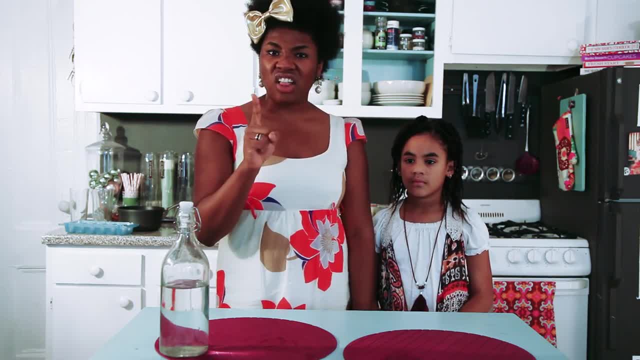 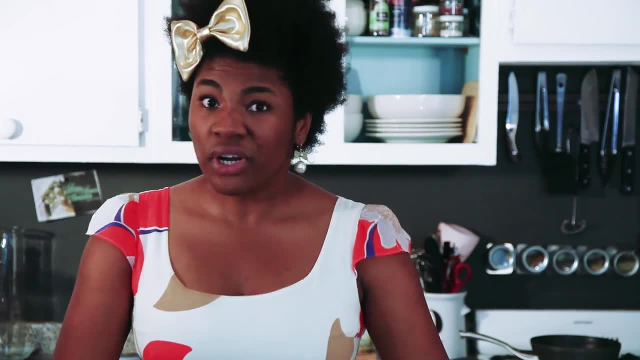 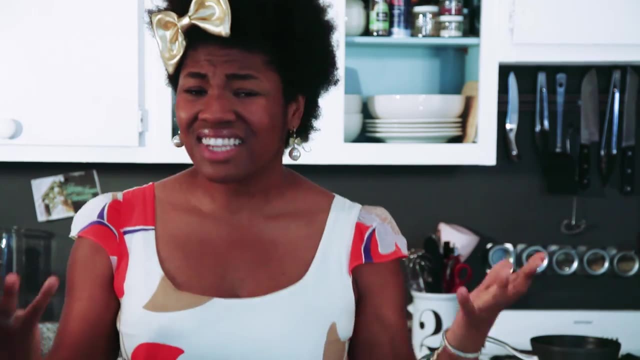 what's the matter? I want you to look them square in the eye and say: solid, liquid or gas. But what about plasma? crazy Aunt Lindsey Plasma, I don't know. it's pretty far out there. It's all about like positive and negative ions and magnetic fields and electricity. 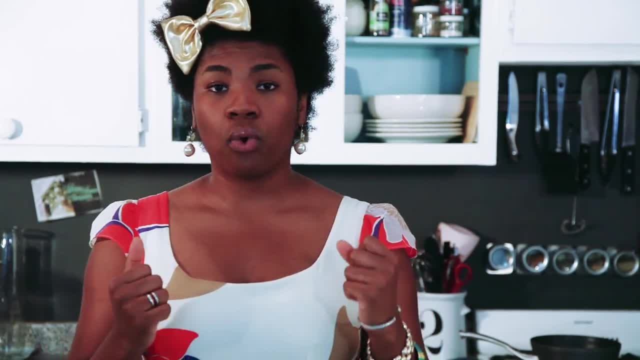 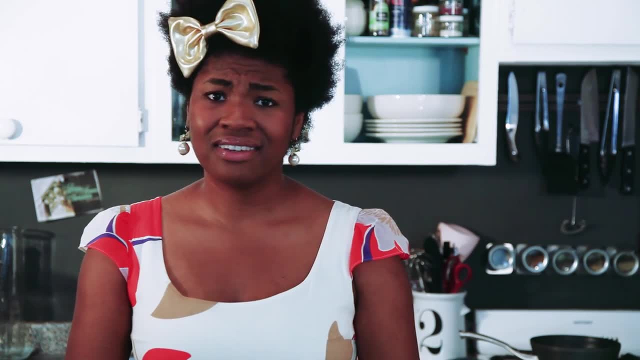 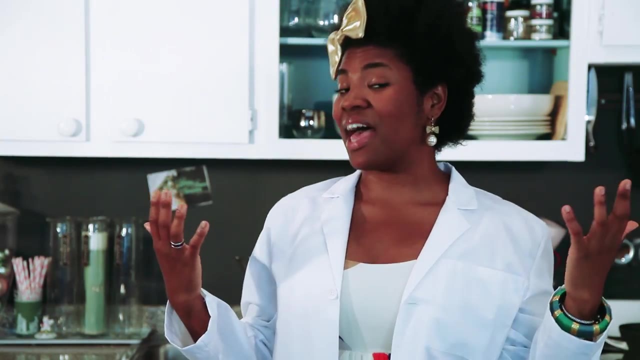 Think the stuff that stars are made of, or the stuff that lightning is made of, or the stuff that's in Nebula And science, I don't know. That's the best I could do. Sorry, I failed to. Now it is time, my friends, for the Fab Lab Wrap Up. 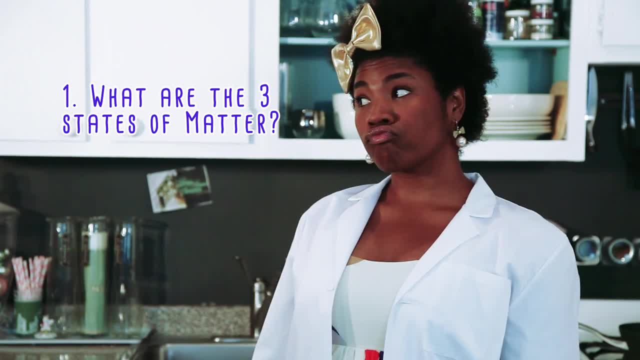 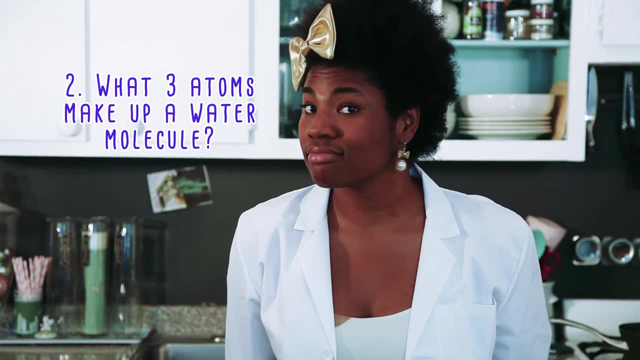 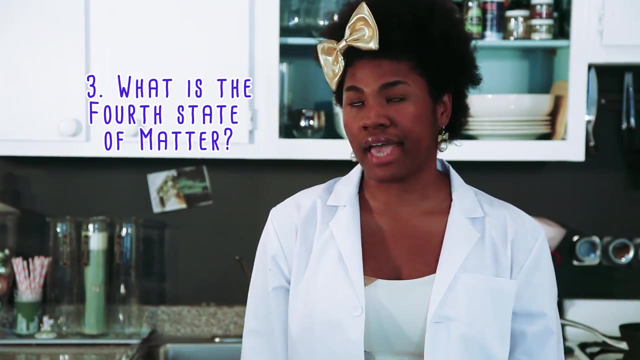 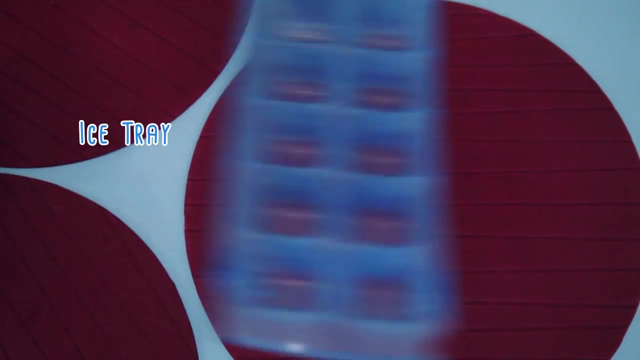 What are the three states of matter? What three atoms make up a water molecule? What is the fourth state of matter that I don't really know anything about? Exactly, That's the science. Now let's make it fabulous. For this part of the project, you are going to need an ice tray. 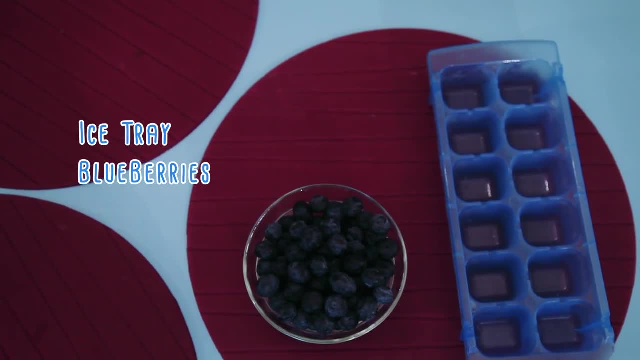 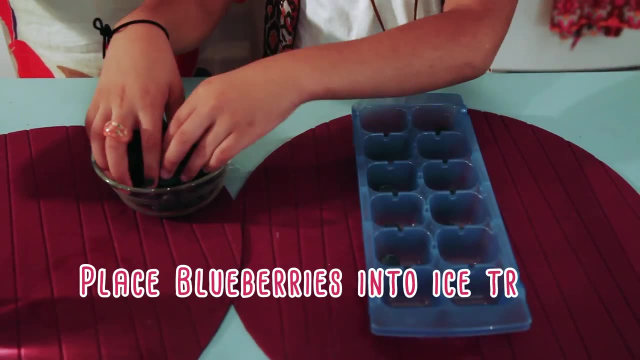 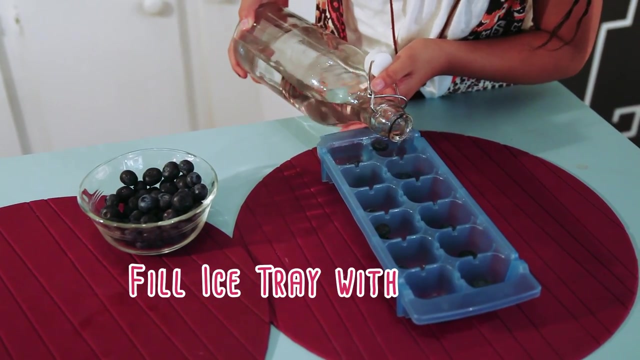 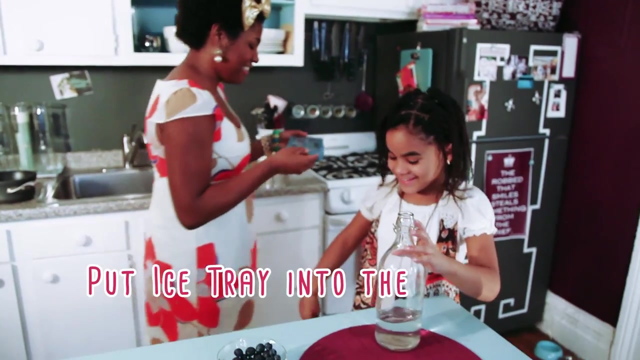 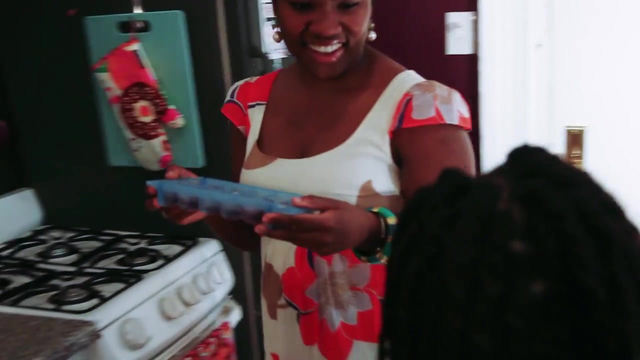 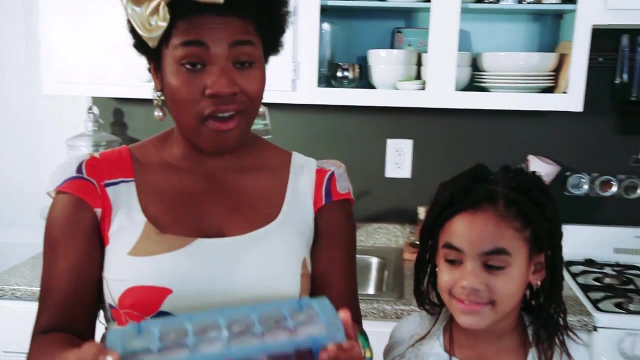 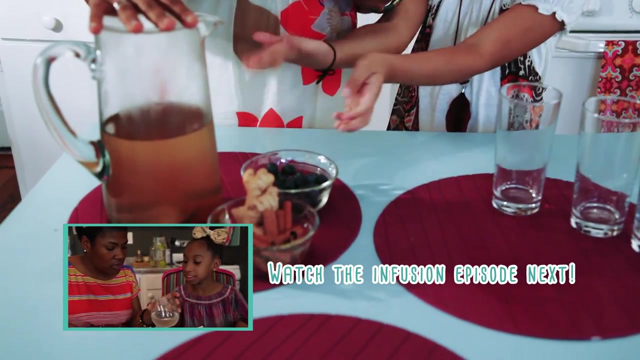 blueberries and water. Woo, Where's the lid? Here it is. Look at how cute they are. All right, everyone. So we have our blueberry ice cubes, which we made to go with our beautiful and fabulous Fab Lab. Cinnamon Ginger Infusion. 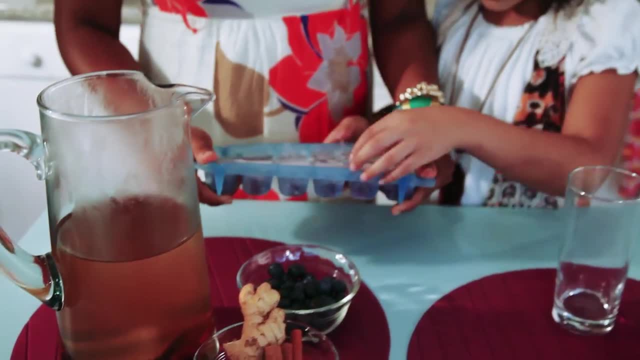 So now we're going to open up our ice Whoa And let's take a look at the bottom. Look, Blueberries. Oh, these are cute. I'm going to just drop them right in. I'm going to drop them in here. 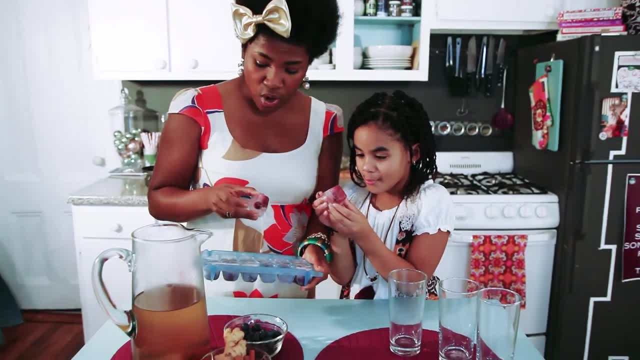 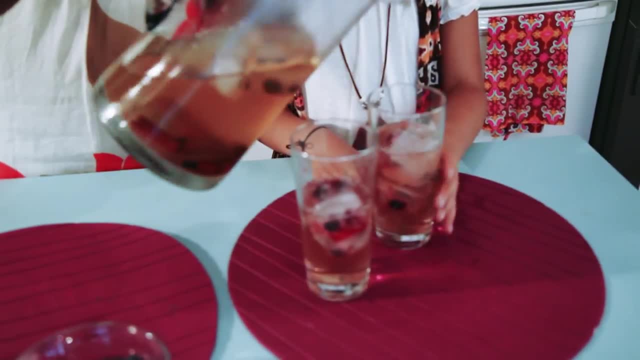 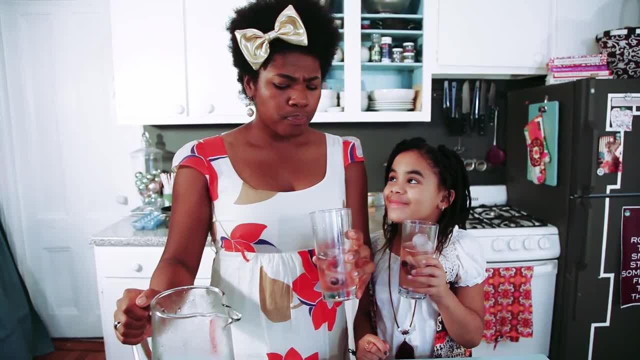 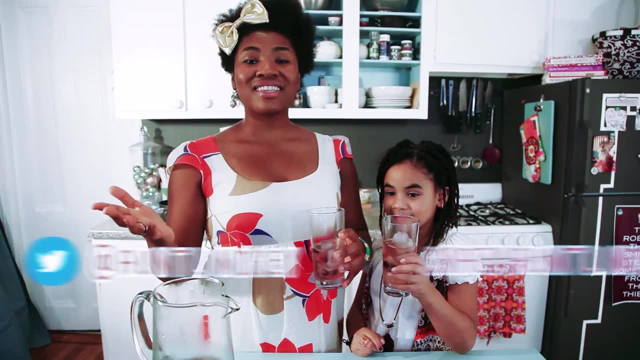 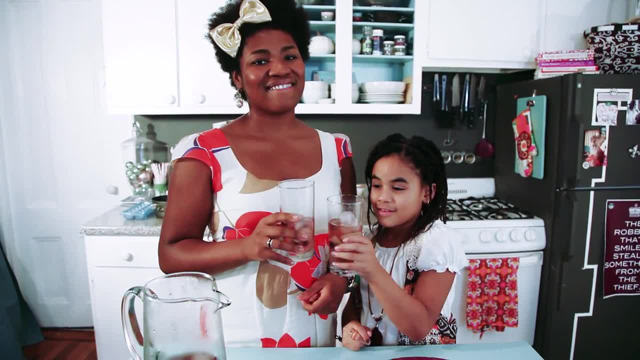 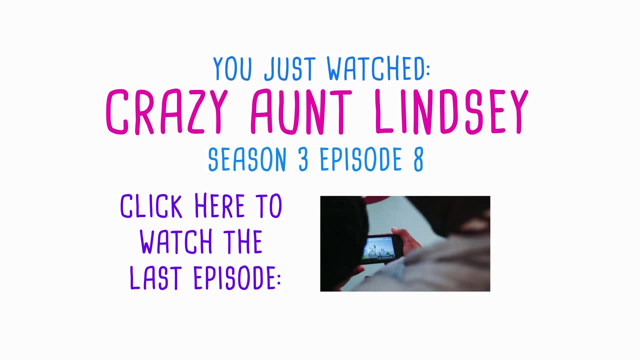